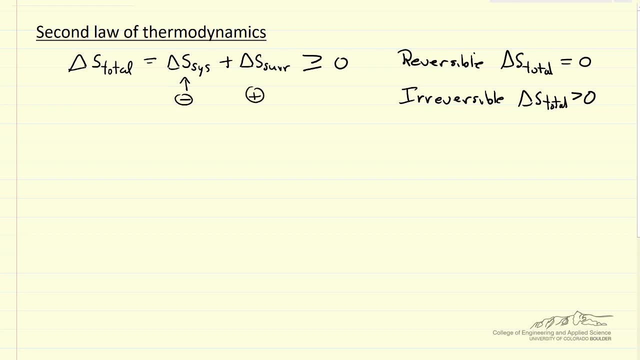 be negative and this number could be positive, and at bigger values. so the sum of them is greater than 0.. Subtitles by the Amaraorg community. So it's possible for a process to have a negative entropy change. If we looked at some specific. 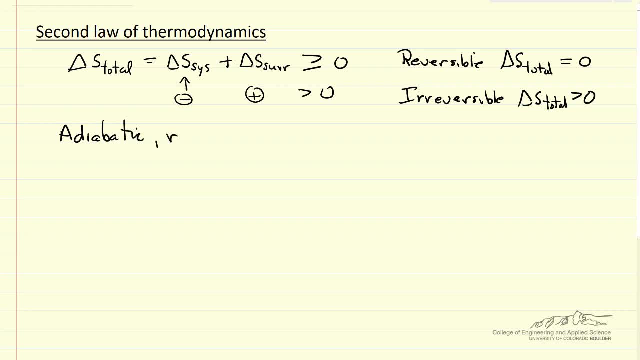 cases an adiabatic and a reversible process. so this means that of course, there's no heat transfer. Q is 0, and if we look at our definition for the system DQ- reversible over T- that's equal to 0, and there's no heat transfer. 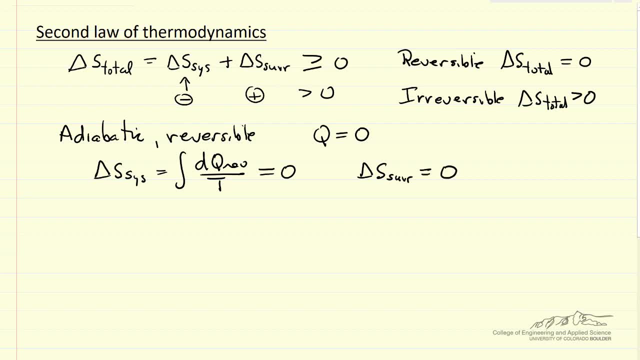 If we look at an adiabatic, irreversible process, delta S of the system must be greater than 0, because delta S of the surroundings is still 0. There's no heat transfer. but the system is irreversible and if we wanted to calculate the entropy change for the system, we'd have 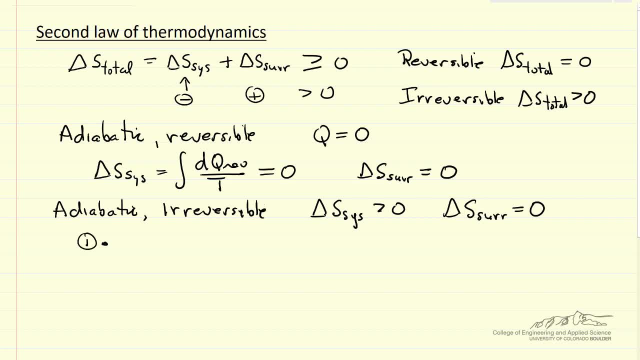 to pick a reversible pathway. So if we're going to from state 1 to state 2 by some irreversible pathway, we want to pick reversible pathway and calculate the entropy, the heat transfer for the reversible process and therefore the entropy change for the system since entropy. 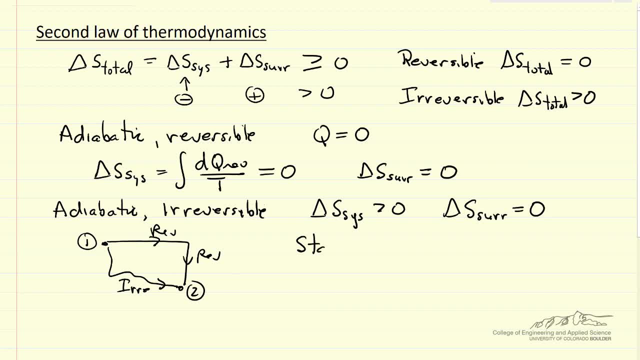 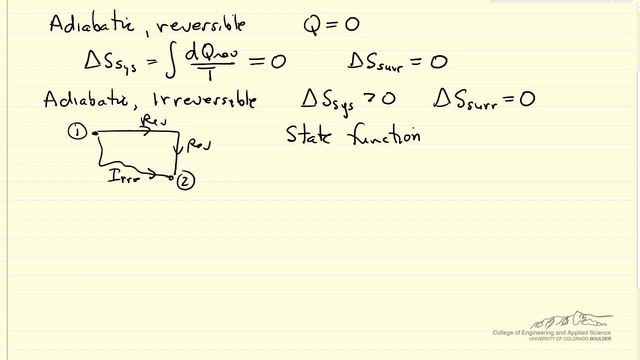 is a state function, So it's important to keep that in mind. entropy is a state function, so we can pick a pathway to make the calculation. Now, if we have an irreversible process where we have just heat transfer to the surroundings, constant temperature, then delta S for the surroundings can be Q over T, where T is absolute. 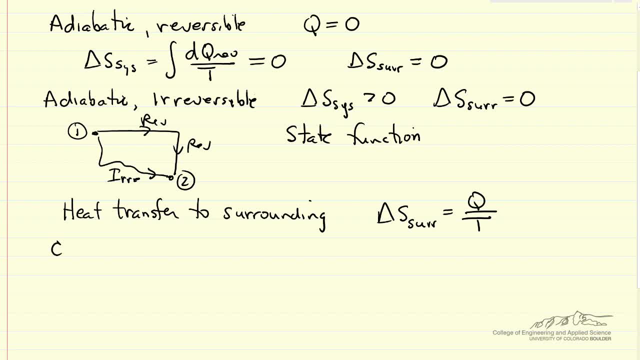 temperature, even if Q is irreversible. Another situation we want to look at is if we are running a cycle, and by this we mean we're running a steady state. So if we have some process running a fluid around continuously in a cycle, nothing is. 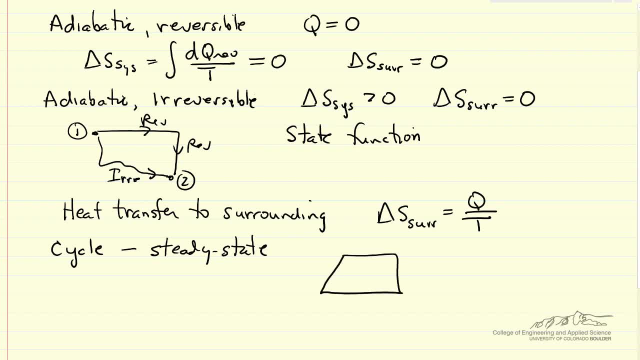 changing in the system. So if we have some process, we look at any point in the system, nothing's changing. So S is constant at this point and what this means is for the cycle then nothing's changing. So delta S for this cycle is 0.. 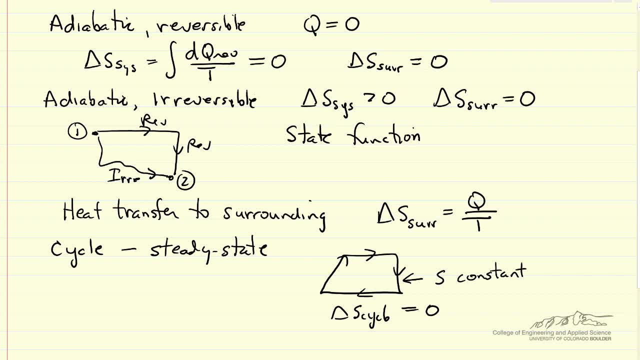 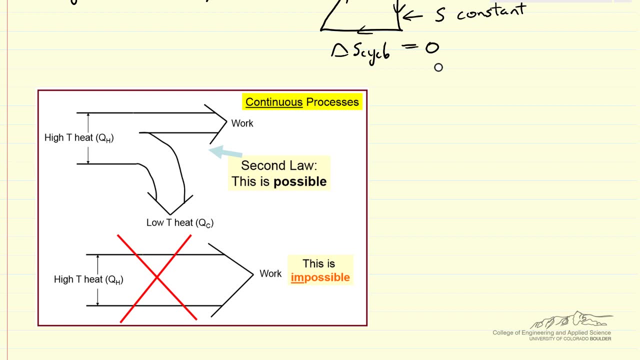 Now it can be transferring heat to and from surroundings. So delta S for this cycle is 0. So entropy change can be positive for the surroundings, but the actual cycle there's no entropy change. So finally, let's look at some an implication of the second law of thermodynamics. 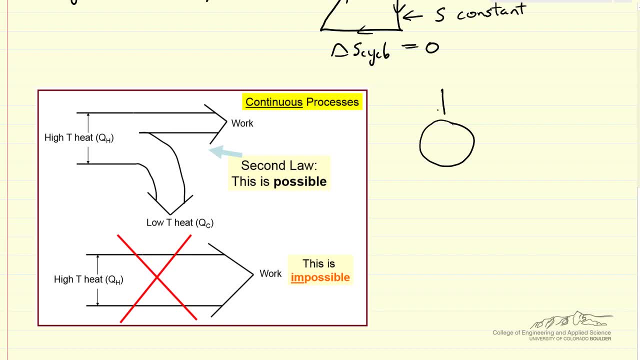 What this says is, if we have a process- we're transferring heat from high temperature and we're getting work out- We also have to transfer heat to high temperature, Heat to a low temperature. So, for example, high temperature, low temperature. 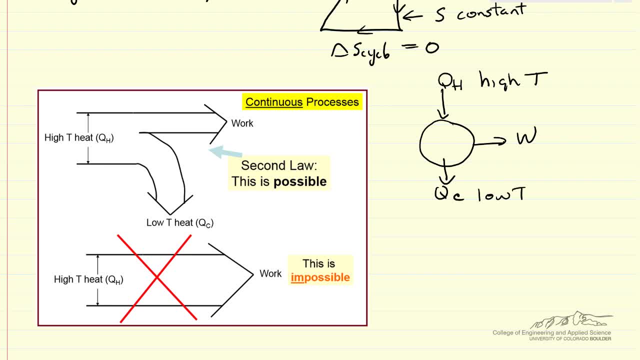 And so if we do this, the entropy change is positive for this process. What we cannot do is transfer heat- and we're talking about continuous process- and just get work out. In other words, we cannot convert heat completely to work, because if we're running it as continuous- 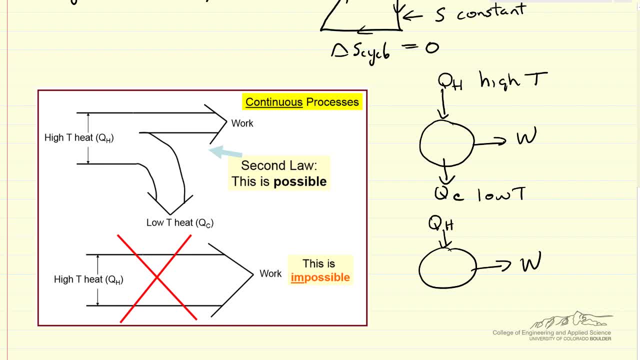 then the entropy change of our system is 0. So we have to transfer heat to a low temperature. So for example, high temperature, low temperature Heat to 0. Entropy change to the surroundings where we transfer heat from is negative. 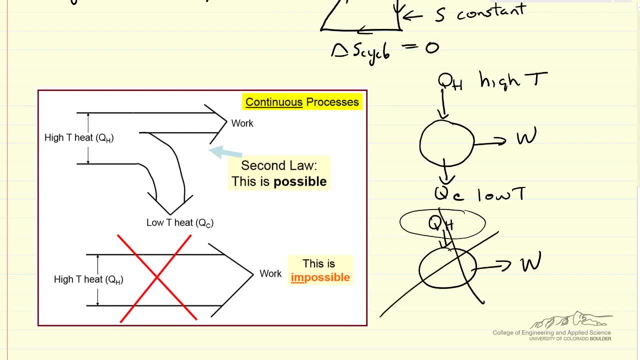 So the overall entropy change is negative. So this is not possible, And so the second law allows us to predict which processes are possible to do. It doesn't tell us how to do them, but it does allow us to predict if a process is possible. 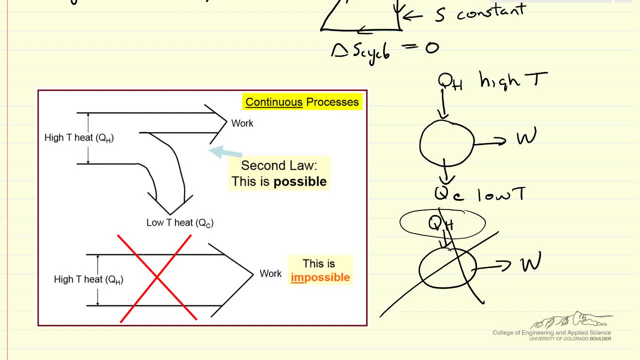 Process would have to satisfy both the first law and the second law, But every process would run through its own boundary, Because this is really one of the order of constants that we want to process. This first is cruel right, And that's what I mention here. So let me tell you about this first thing. So each matrix, this first matrix, for example, with your block closed off, it's called the two-. элемents. the two complements are two-elements, So they're start and finish. So these two complements are the two-element that can do the work. So those дв- east양 and the north-eastang are the two-element cast minus beams. Souzu is coming, And so that is the push spurt of all the paramètres. So congratulations to that Clean heat. let's just call it Machado kissing the swell this cool workroom here.